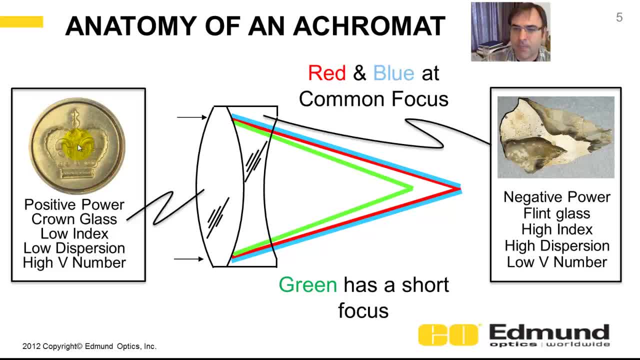 Now crown glass. if you recall from the last optics lecture, it got that name because it was plate glass that was blown and flattened in the center where the pole stuck into it They would stamp. They would stamp with the royal seal, which was a crown. 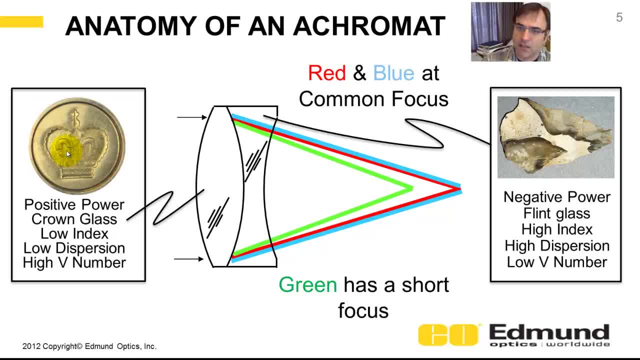 Crown. This glass is usually lower index. It's got lower dispersion or high V number, high Ave number. Remember those two are inverse of one another, dispersion and Ave number. And a flint glass is negative power. It's going to have a high index. 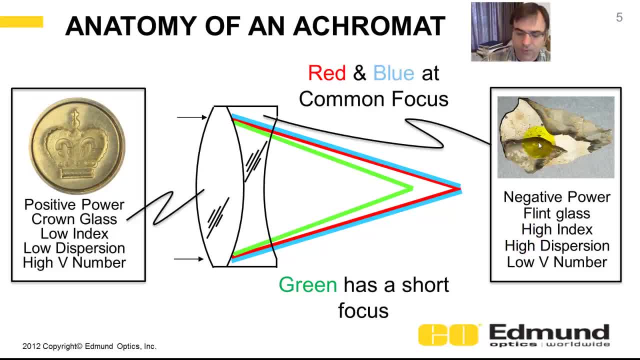 Normally they're higher index, higher dispersion And flint because they the original form of it. they used flint rock out of the river, the riverbed, to create it. Today we use we tend to put lead and other interesting materials. 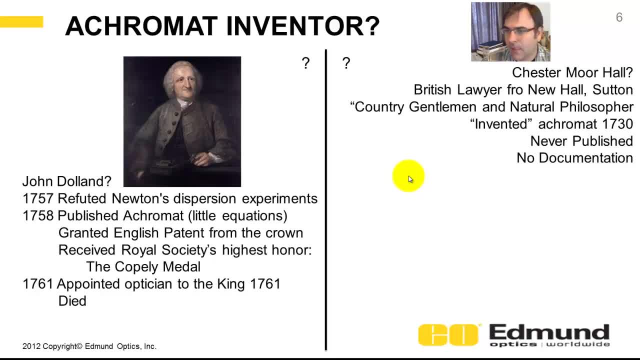 in to dope the glass, to give it that high dispersion. I just briefly want to touch on the history. So who invented the acromat? And there's two versions of history and it appears like we really don't know who made it. So on the left side, here we have John Dolan. 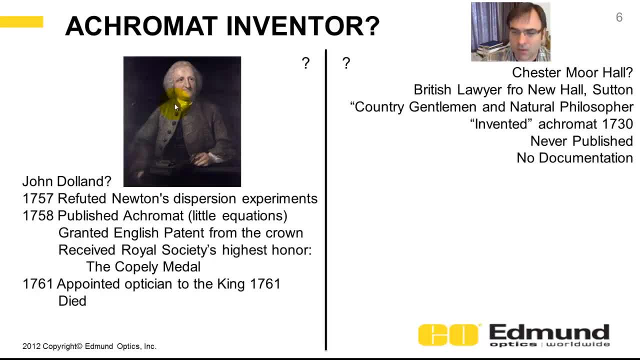 He on paper. he got the patent, he, you know, in theory he's. he is credited with the invention of it. If you recall, in 1757, he refuted Newton's dispersion experiments And in 1758, he published about the acromat, with very little equations. 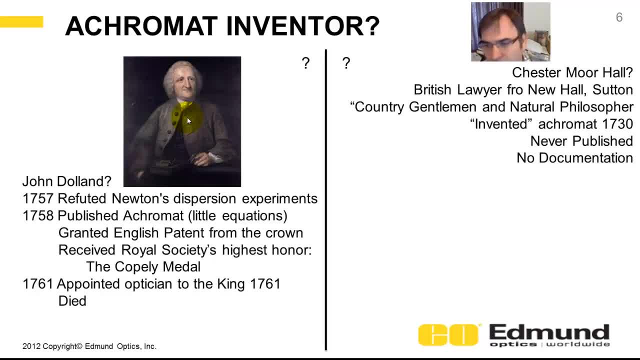 He got a patent that year and he received the Copley Medal from the Royal Society And he died soon thereafter and he was appointed optician to the king. So that's on one side of the argument. The other side of the argument is that it really was invented. 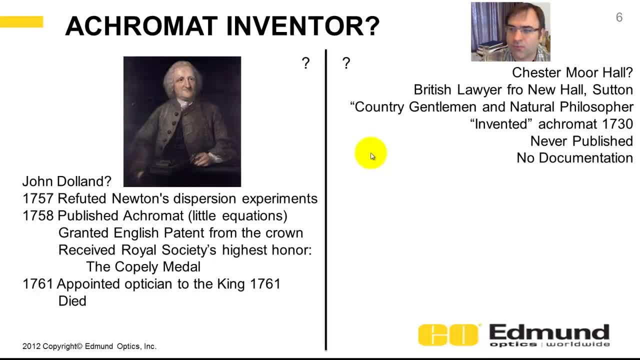 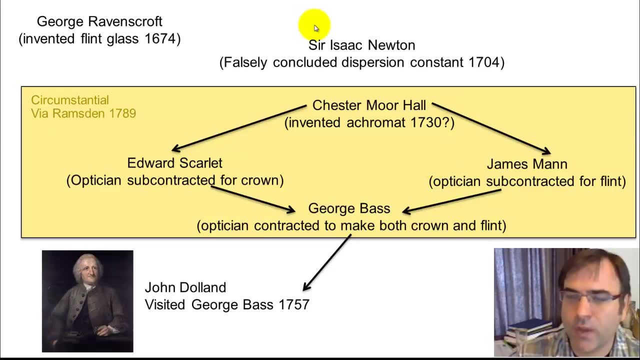 by Chester Newton. It was invented by William Moore Hall, who was a gentleman, you know, country gentleman, natural philosopher, that was a little secretive about what he did or not open about it. He never published, There was no documentation. So here's just a quick summary of the invention of the acromat. 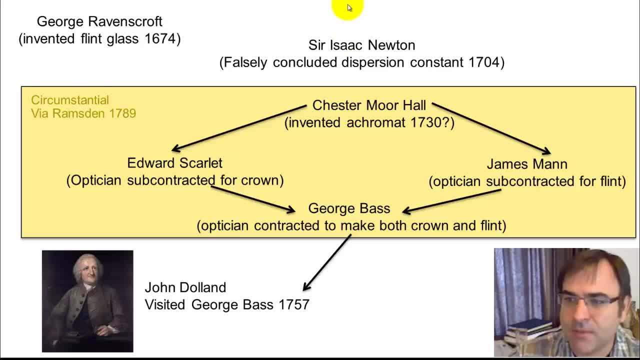 To me this is really, really fascinating. And time is in the vertical axis, So we've got early time here and late time at the bottom. Recall George Ravenscroft: He invented flint glass by doping it. going away from flint rock, river rock. 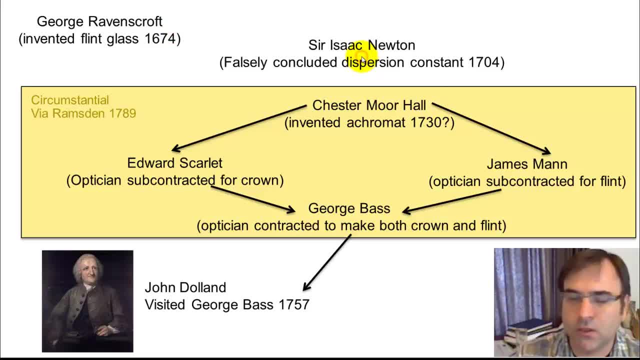 and putting lead glass into it. And Sir Isaac Newton? he concluded incorrectly that all dispersion in glass was constant in 1704, pretty much because his instrumentation wasn't good enough. Now this yellow box here is circumstantial. It's not clear if this is the history. 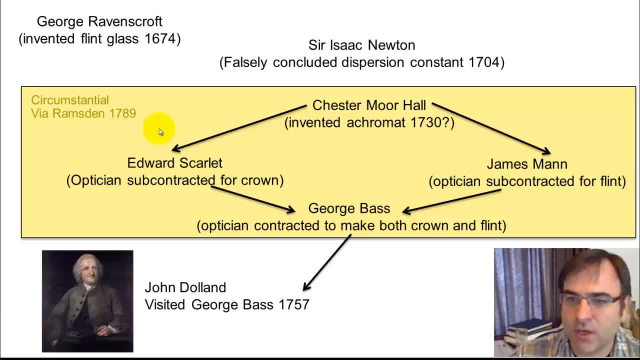 It's not clear if this is the history historically. this is historically accurate. This is credited to Ramston in 1789, and we'll talk about him on the next chart. So the flow of events was that Chester Moore Hall invented the acrobat. 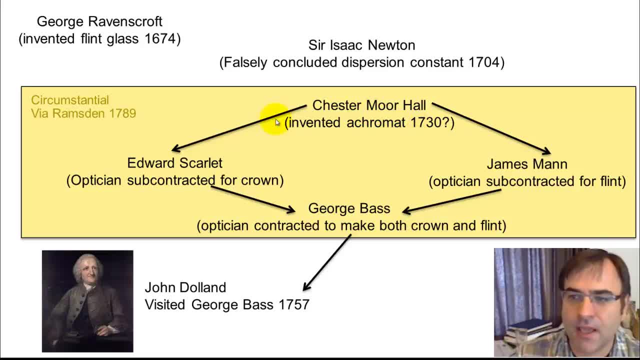 sometime in 1730.. And to keep it secret, he gave one glass to one optician and then the other glass element to another optician. Now I just, you know, supposed here Edward Scarlet. one optician got the crown and James Mann got the other a flint. These two men happened to subcontract. 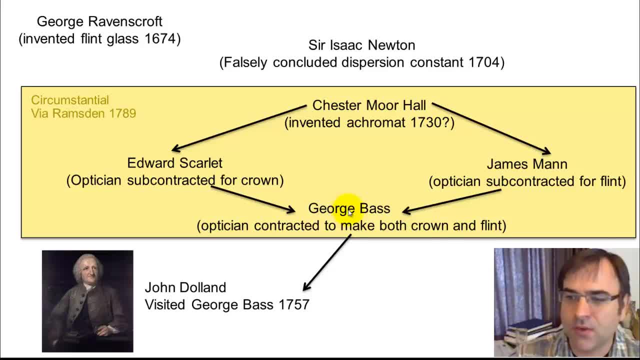 to George Bass And either he or John Dolan figured out that those two radii at the interface are matched. Now it's documented that, George, that John visited George Bass in 1757. So maybe John Dolan got the idea from there, Maybe he, you know, who knows? After John Dolan's death, 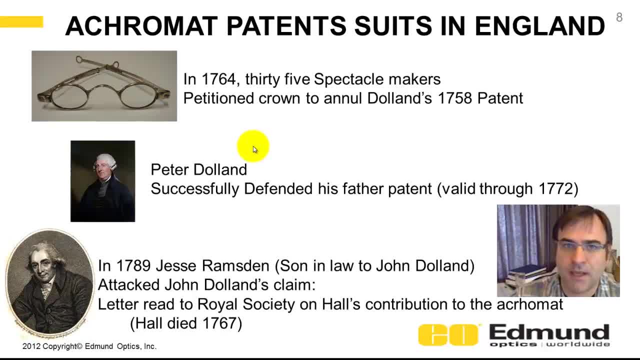 a lot of London opticians started making acromats And of course it was patented. They had to pay royalties And this you know. at the time it was spectacle makers that were making land surveying, optical instrumentation, telescopes and microscopes. So in 1764, 35 spectacle makers. 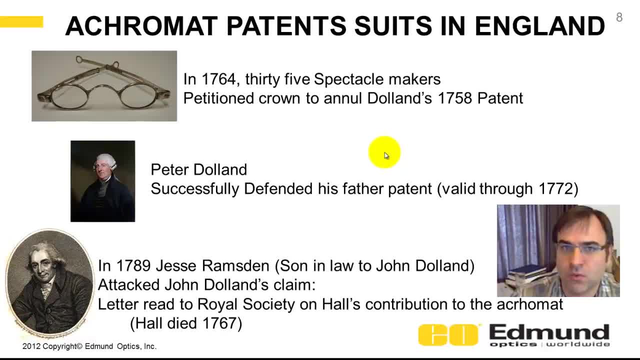 came together and they petitioned the crown to stop Dolan's 1758 patent. Now, at this point, John Dolan had passed away and his son and business partner, Peter Dolan, successfully defended that patent, which was valid till 1772.. Now, Peter, at that, you know. 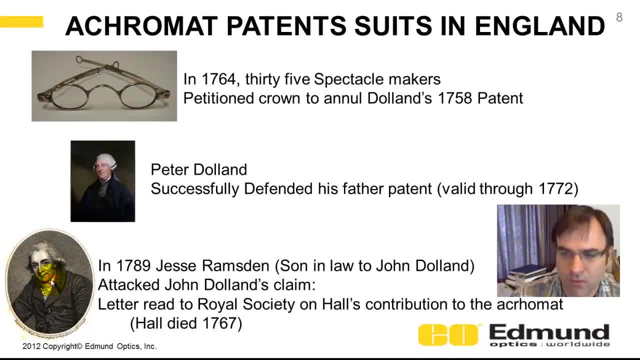 fighting off the spectacle makers actually was joined with his brother-in-law, Jesse Ramston, But in 1789, he attacked John Dolan's claim by reading a letter to the Royal Society on Hall, Chestermore Hall's contribution to the acromat. Now, Hall had died previous to this And it was a very persuasive. 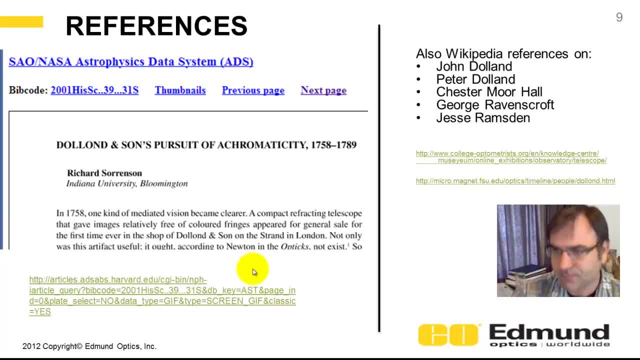 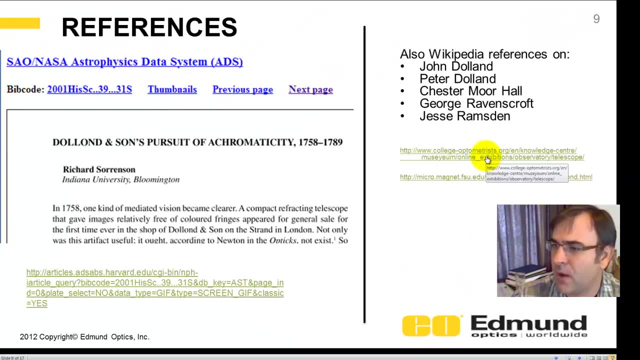 letter, but we don't know if it's historically accurate. Here are my references. I get the majority of it from the harvardedu, this article from Richard Sorenson out of Indiana University, as well as Wikipedia and some optometry and some other websites here. So how does an acromat 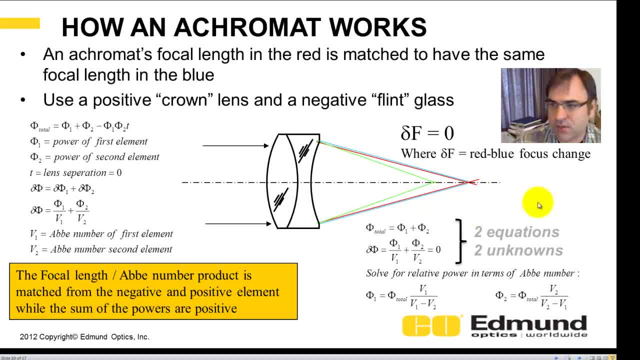 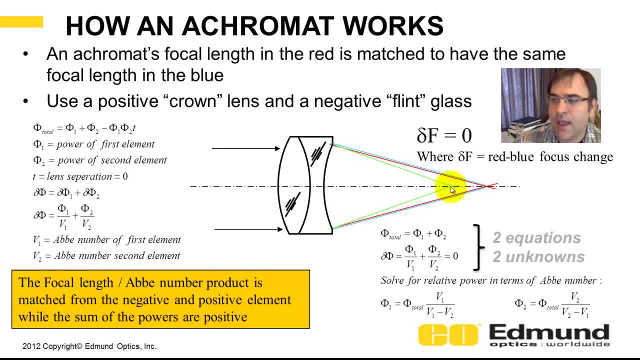 this is really. this is here's the equations. Now, recall, an acromat will put the two wavelength extremes, red and blue here and the middle green at some other focus. So we'll start with the total power for the lens, which is actually going to be the power of the crown, phi 1,. 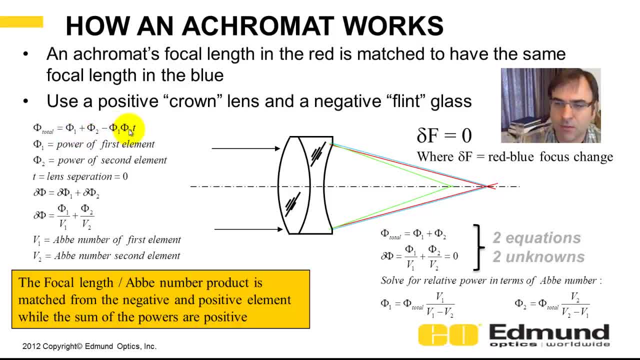 plus the power of the flint phi 2, minus their product times, the thickness. Now, each of these is going to have a principal plane and there is going to. even though they're cemented, there's going to be some thickness. 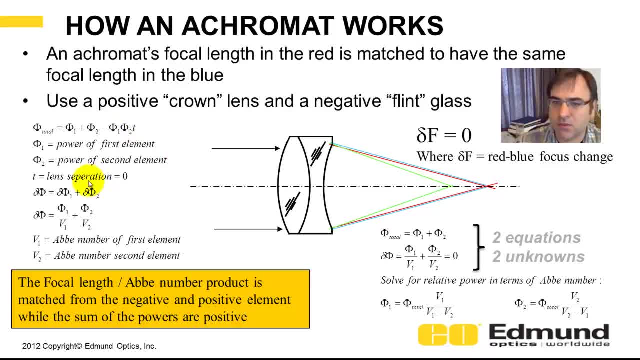 here. For sake of argument, we're going to assume that lens separation is zero And from last tutorial we found that a single lens's axial color is proportional. the change in focus, change in power is proportional to phi 1, proportional to its power divided. 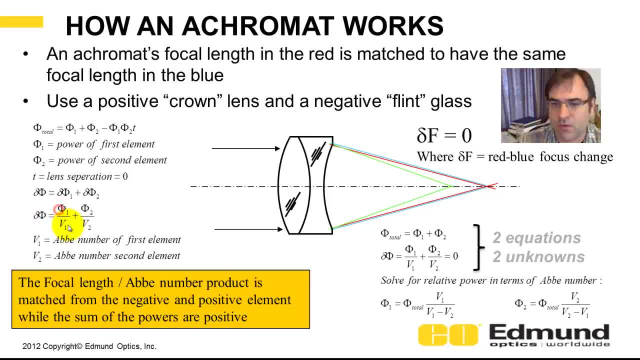 by its Ave number. So for this lens the total dispersion is phi 1 divided by V1, plus phi 2 divided by V2.. Now we've got two equations: power and setting the total color to zero. Two equations, two. 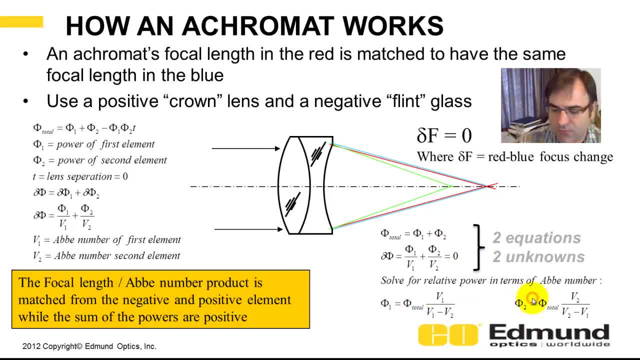 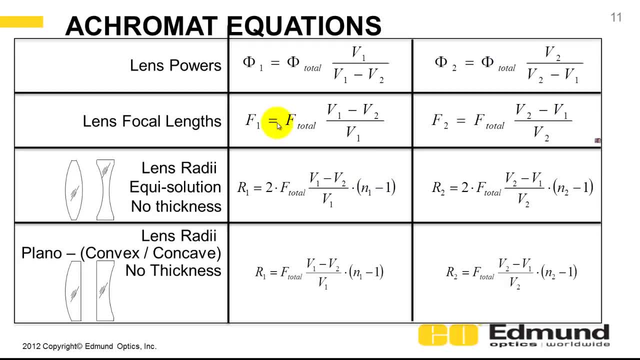 unknowns, You can solve for the power of the crown and the power of the flint. Now I've rearranged these, if you look at it slightly differently. So the first row is based on power from the last chart. If you prefer to work in focal length, it's really the inversion. 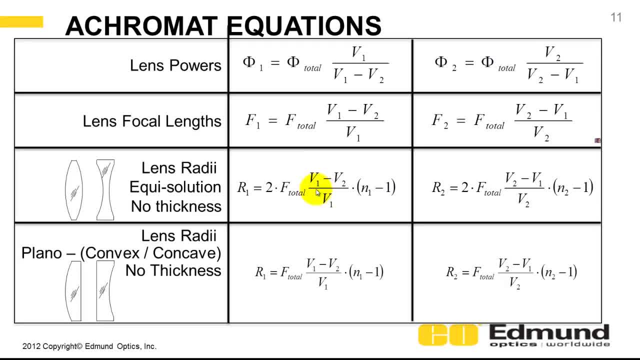 of that. If you're going to enter these into a ray trace code, you need to enter radii. So I've solved for what radius you need, assuming an equiradius solution, bi-convex, bi-concave, and it's this third row here. 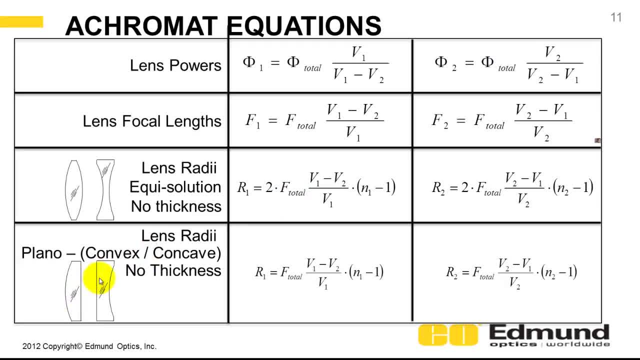 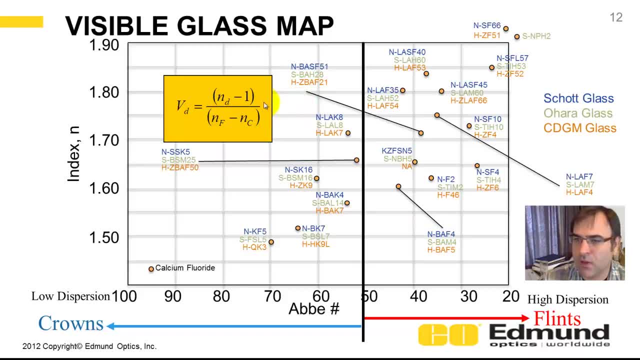 Or, if you wanna do, a plano-convex concave lens, and it's this radius here, so it's a factor of two Here, and this is from last time as well. this is a glass map and this is showing index. 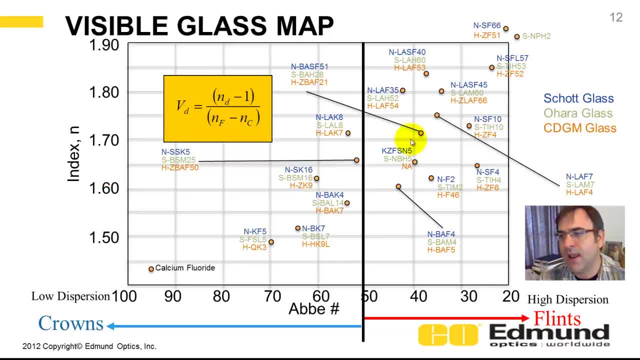 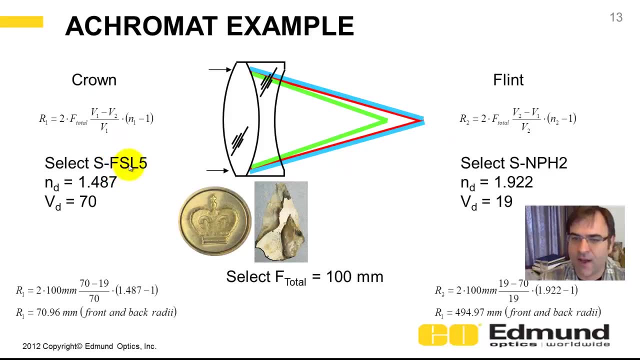 in the vertical, dispersion in the horizontal, and I'm doing it for three different glass types. I think next tutorial we'll discuss some of the makeup and what's in these materials. Here's an example: let's do a crown of SFSL5,. 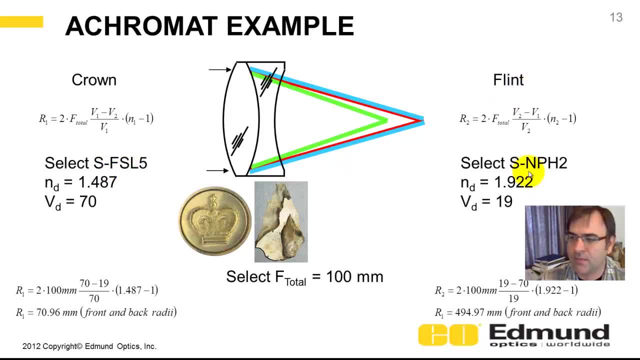 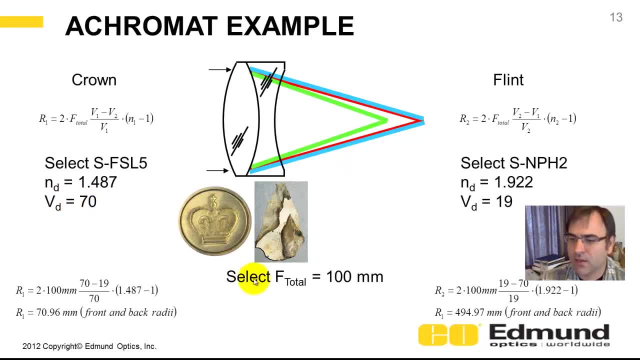 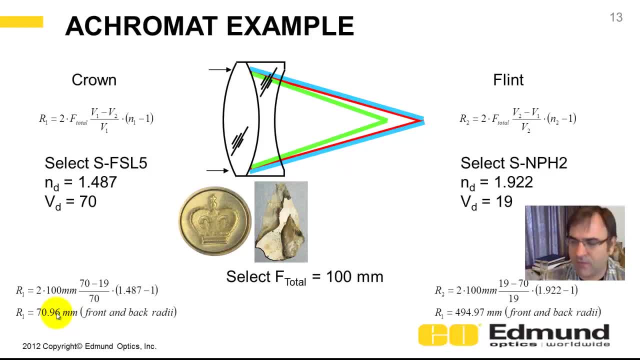 The crown has a 71 millimeter biconvex and the flint has a 495 biconcave solution. If you enter this, if you try to enter this in a ray-trace code, make sure to start with a zero thickness, otherwise the color solution. 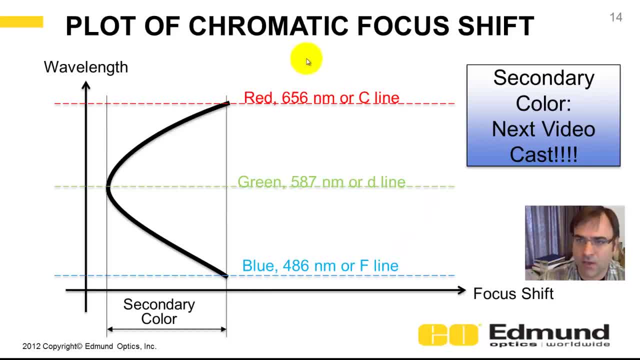 probably won't come in. How do we look at color? Well, if you plot the focus versus wavelength, you get this chromatic focal shift. So in the vertical we've got wavelength, in the horizontal we've got focus shift. 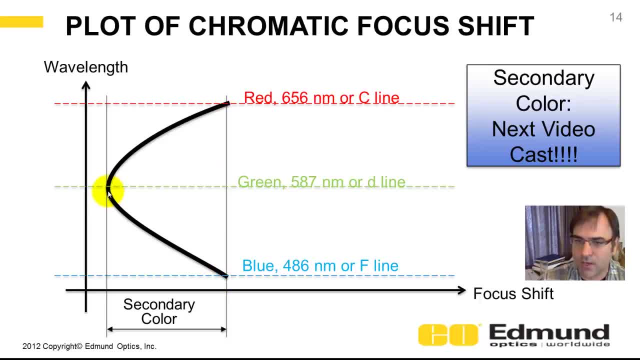 And you can see the blue and the red come to a common focus and green is out here at some other focus. The distance between these two, from green to the common blue-red is referred to as a secondary color. Next Optics YouTube lecture. I'll go into talking about that. 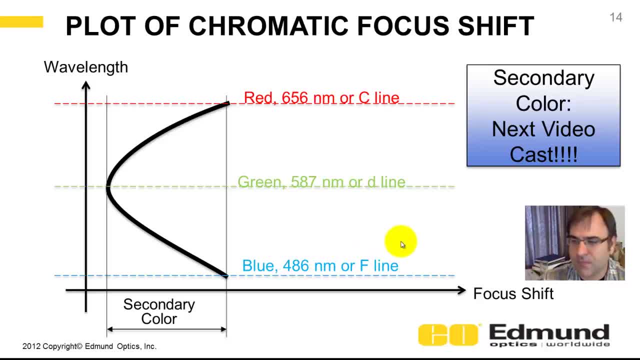 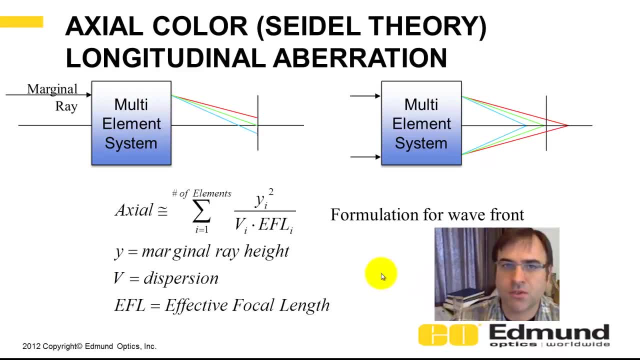 how to compute it, what it means and how to minimize it. Finally, I want to briefly touch on Seidel aberration theory Seidel constructed. he shows how to compute for a complicated optical system up to Third Order aberrations, And I just briefly wanted to simplify that. 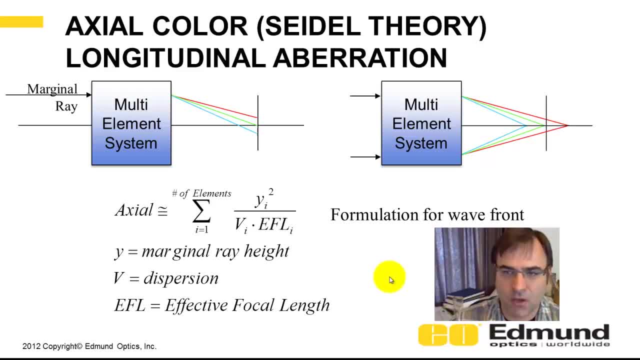 and show it for axial color. Now, really, Seidel, he did this on a surface-by-surface basis, but we'll look at this for sake of clarity. we'll look at it based on elements, so the axial color is proportional to.